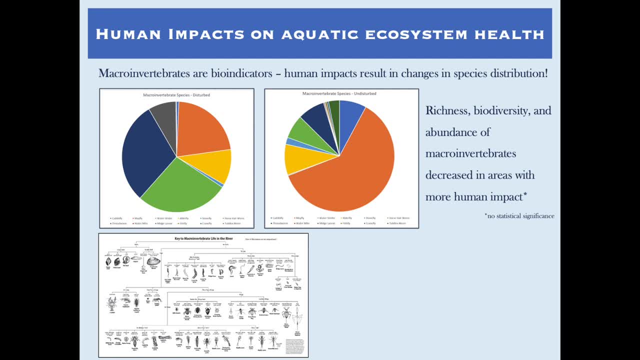 in Sandstone Ranch to support diverse and abundant macroinvertebrate populations. We examined both undisturbed sites in which human impact has been minimal to none, as well as locations that have been altered by humans, including a dam site and a gravel dumping. 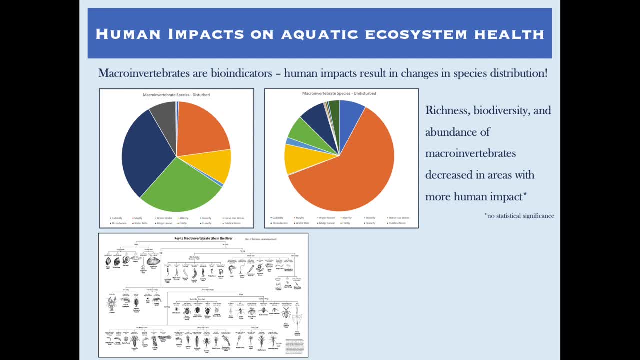 site. We hypothesized that human disturbance of an aquatic ecosystem affects water quality and macroinvertebrate biodiversity, and we predicted that areas of aquatic ecosystems that have been disturbed would have differing depth levels that cause unnatural flow and poorer water quality, and therefore have less macroinvertebrate biodiversity. 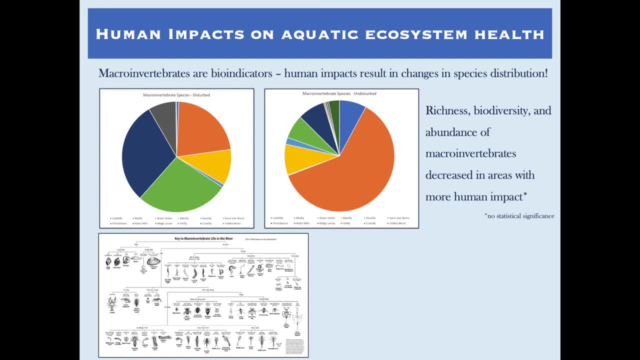 than undisturbed areas. After data collection, we conducted several different types of statistical analysis to determine significance. First, we concluded that there was no significant difference in values for pH, conductivity and water quality. We also determined that the water quality of 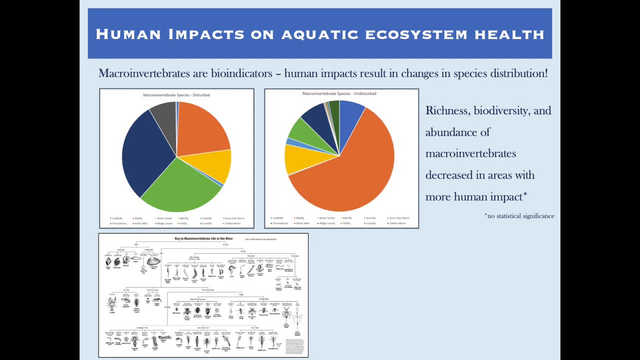 the water is consistent with the water quality of the soil and dissolved oxygen, which signifies that the abiotic water quality indicators are consistent between the disturbed and undisturbed sites. We then analyzed data for the macroinvertebrate diversity and abundance. Pie charts of the macroinvertebrate species found in the disturbed and undisturbed areas can be seen. 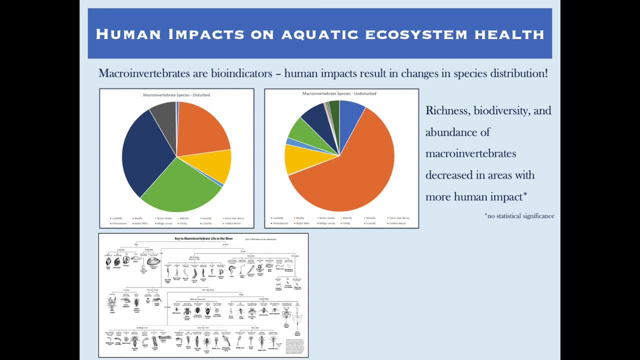 on the poster. The major findings from these charts were that there were many more mayflies in undisturbed areas and that there were many more horsehair worms in disturbed areas than undisturbed areas. This was interesting, as mayflies are considered to be indicator species as they are very sensitive. 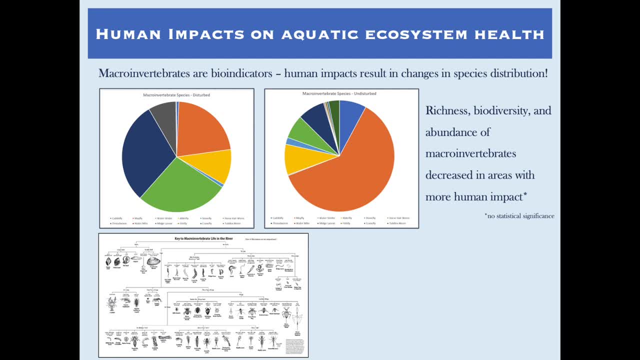 to environmental disturbances. We continued our macroinvertebrate analysis by conducting a test that accounts for both diversity and abundance of species. We found that the values for diversity and richness were larger in undisturbed sites than disturbed sites. However, statistical analysis showed that there was no significant difference between the disturbed 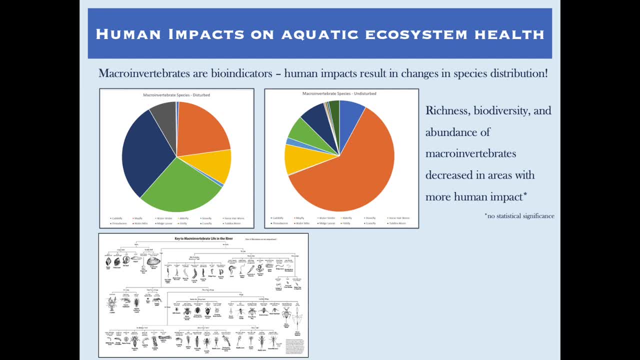 or undisturbed sites. In conclusion, our hypothesis was somewhat, but not fully, supported, as we were not able to determine the differences between the disturbed and undisturbed sites. In conclusion, our hypothesis was somewhat, but not fully, supported, as we had a large 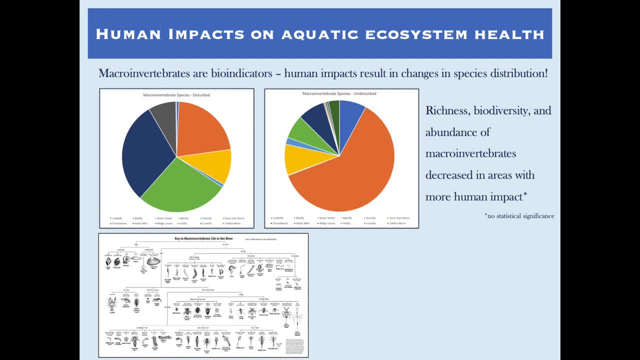 number of data from the undisturbed and undisturbed sites and we were able to determine the, as there was no statistically significant difference between water quality or macro invertebrate diversity and abundance between the disturbed and undisturbed sites. However, our data suggests that there might be a difference in macroinvertebrate diversity if more data was.